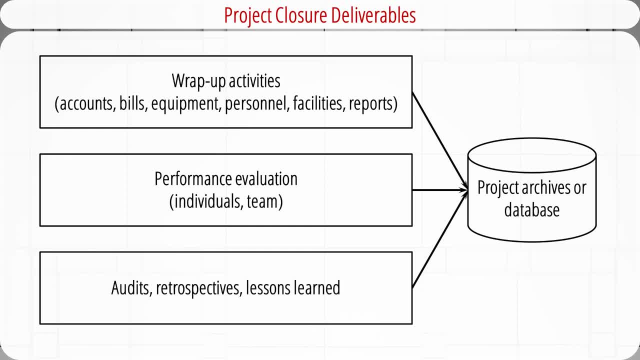 Audits and retrospectives are post-project reviews to see how successful the project was. The outcomes of all these tasks will go to the project archives or database to provide important information for future projects. There are five different types of project closure. Normal closure means the project. 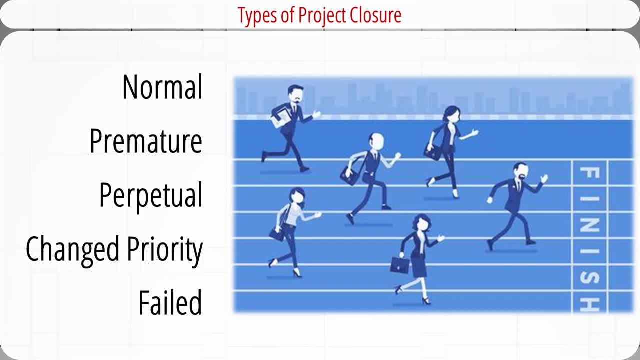 ended successfully. For development projects, the end involves handing off the final design to production and the creation of a new product or service. For IT projects, like system upgrades or creation of new inventory control systems, the end occurs when the output is incorporated into ongoing operations. 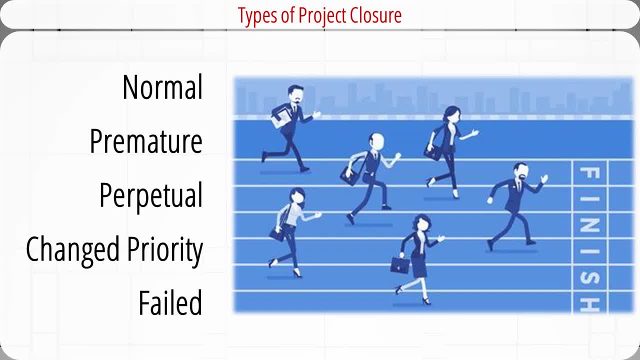 Premature closure means the project may be completed early, with some parts eliminated. For example, in a new product development project, a market manager may insist on releasing products before testing. Perpetual projects are those projects that never seem to end. Constant add-ons suggest. 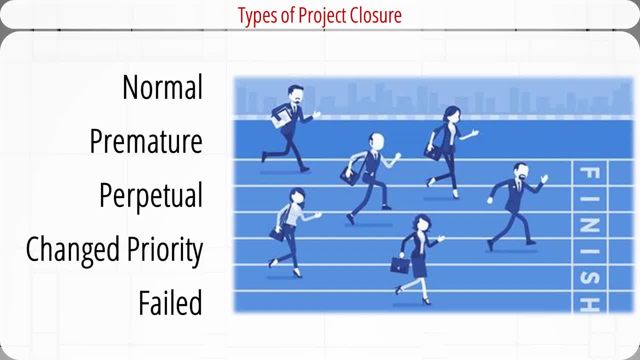 a poorly conceived project scope. A good strategy to deal with a perpetual project is to bring the project to a closure and initiate a new project for significant add-ons. Organization's priorities often change. For example, during the 2008-2010 financial crisis, organizations shifted their focus. 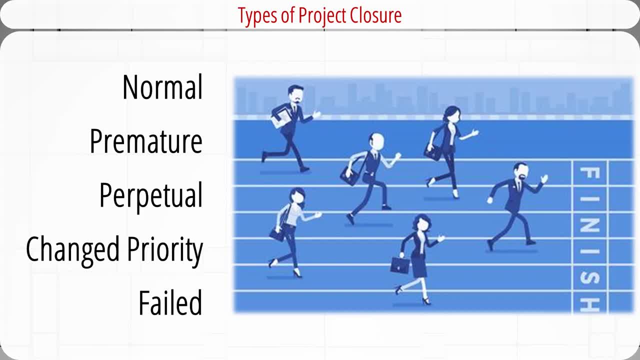 for money-making projects to cost-saving projects. Therefore, a project may start with a high priority but see its rank erode or crash during its project life cycle as conditions change. When priorities change, projects in progress may need to be altered or canceled, For example. 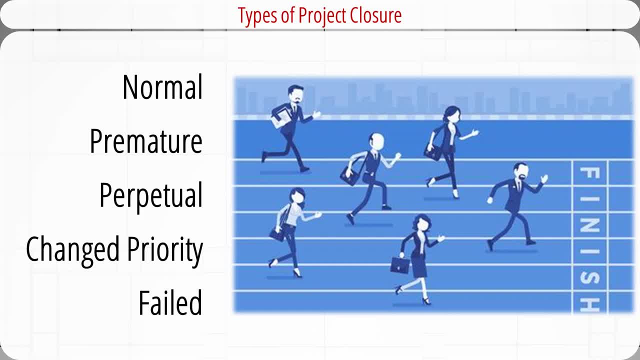 a new project may be completed early, with some parts eliminated. A good strategy to deal with a perpetual project may be to bring the project to a closure and initiate a new project for significant add-ons. This is another form of project closure. The final type of project closure is a failed project. Some projects fail because of lack. 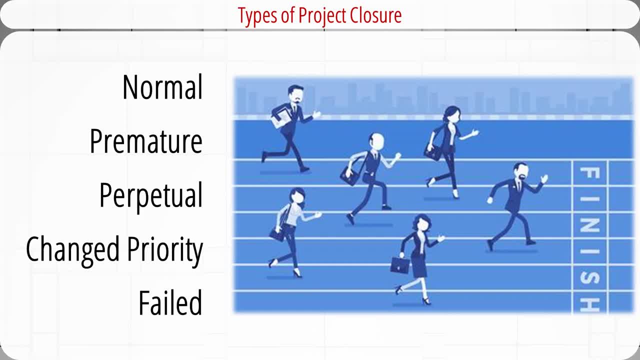 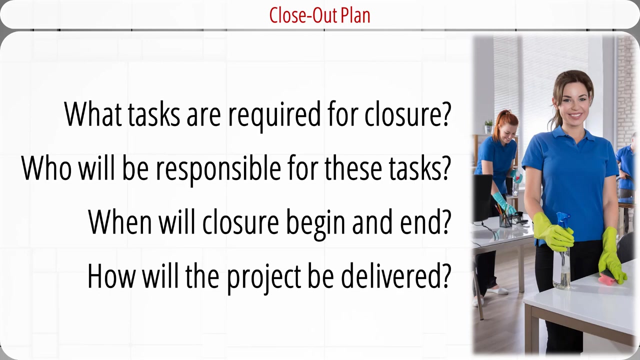 of management skills of the project manager or lack of technical skills of the team members. Other projects fail because of situations beyond the control of the project team. For example, a competitor released cheaper products. The project manager's challenge is to keep the project team focused on the remaining activities. 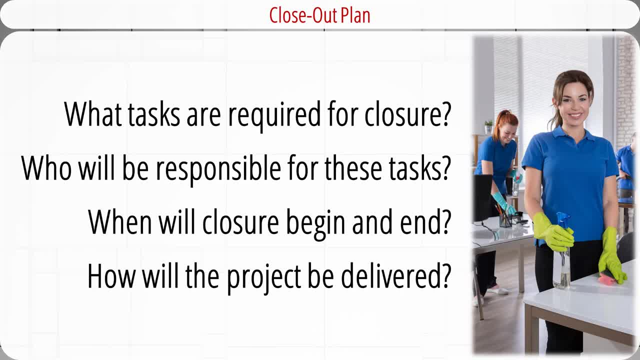 and deliver it to the customer. until the project is complete, The manager needs to communicate a closeout plan to allow the project team to accept the psychological fact the project will end and prepare to move on. The closeout plan should answer questions like what tasks are required to close the. 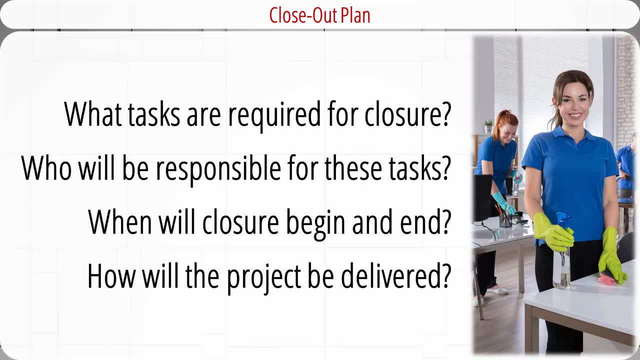 project. Who will be responsible for these tasks, When will closure begin and end, And how will the project be delivered? It's like the party is over now who wants to help clean up, And much of work at this stage could be mundane and tedious. 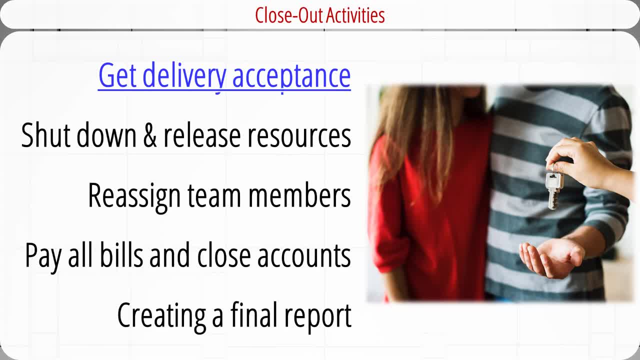 Getting delivery acceptance by the customer is a major and critical closure activity. Customer satisfaction is important. Watch this video to see why. Another important activity is to shut down resources and release them to new use. And then we assign project team members. Releasing the project team members typically occurs gradually during the closure phase. 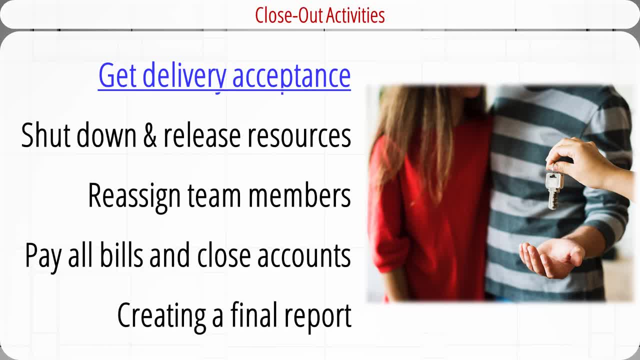 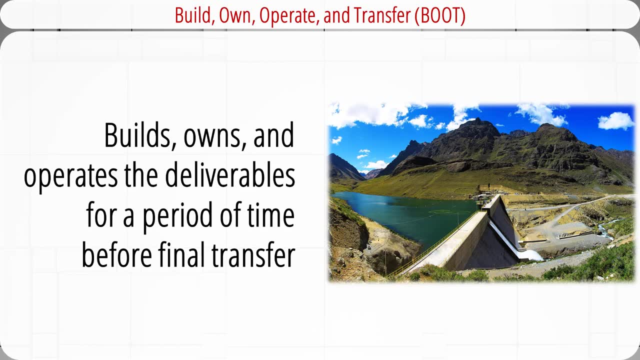 The manager also needs to make sure to close all accounts and see all bills are paid. Finally, a project report is created to conclude the project. For small projects, the project outcome delivery may only take a few hours or a few days. For large projects, the BOOT deliverer approach can be used. 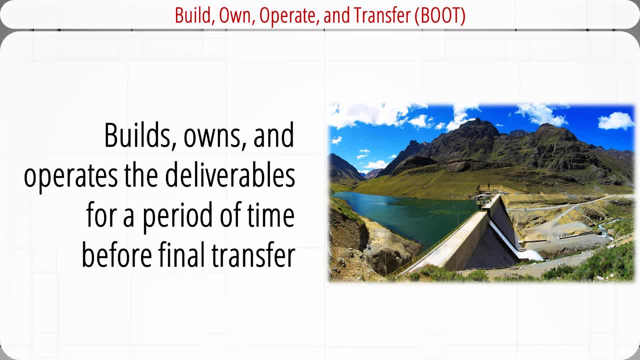 BOOT stands for Build Own, Operate and Transfer. Basically, the contractor builds, owns and operates the project. deliverables: BOOT stands for Build Own, Operate and Transfer. BOOT stands for Build Own, Operate and Transfer. 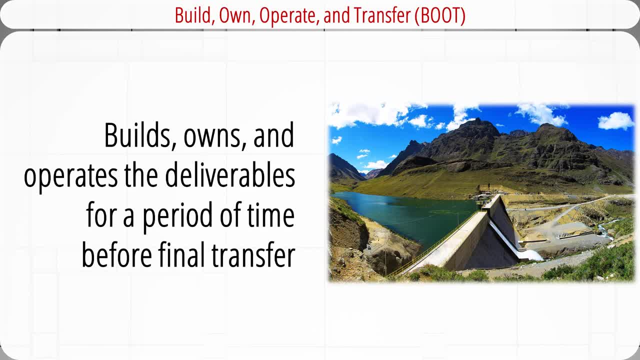 The contractor will deliver BOOT on the project for a set period of time before finally transferring the deliverables to the customer. For example, a company may build a hydroelectric power plant and operate it for six months before turning over operations to their customer. During this time, all the problems are fixed and conditions for final delivery are satisfied. 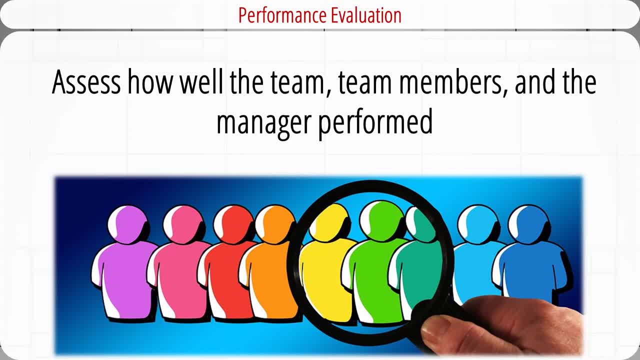 An important task during project closure is the performance evaluation. In the end, a project may be sold after a certain period of time. performance evaluation- Performance evaluation assesses how well the project team, team members and the project manager performed during the project. 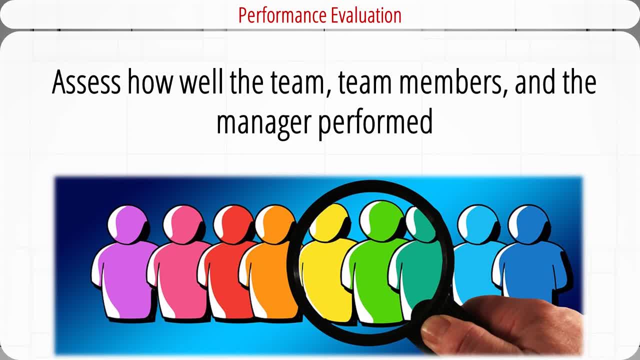 Performance evaluation is also called performance appraisal. It fulfills two functions. One is to identify individual strengths and weaknesses and developing action plans for that individual or team to improve. The other is to assess how well the person has performed in order to determine merit adjustments like pay raise or promotion. 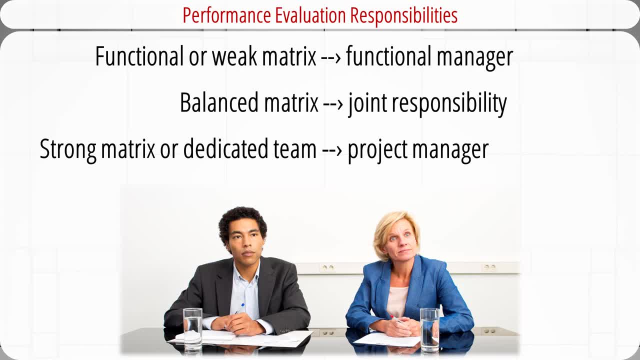 When evaluating team members' performance, the project manager and functional manager may have different responsibilities depending on the organizational structure used for managing the projects. When a project is carried out in a functional organization or using a weak matrix structure, the team members' performance performance may be reduced by one. 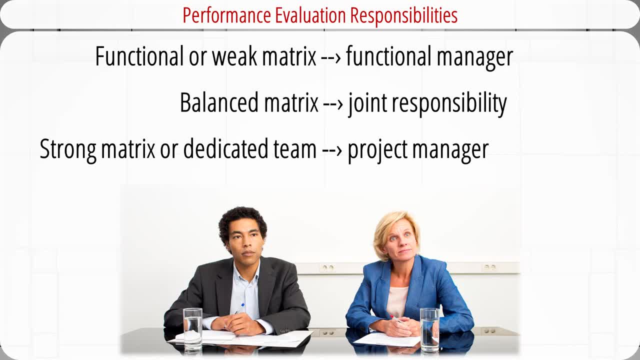 The team member's functional manager will have the main responsibility of assessing the team member's performance on a regular basis. The functional manager may solicit the project manager's opinion of the individual's performance on a specific project. When the balanced matrix structure is used, the project manager and the functional manager 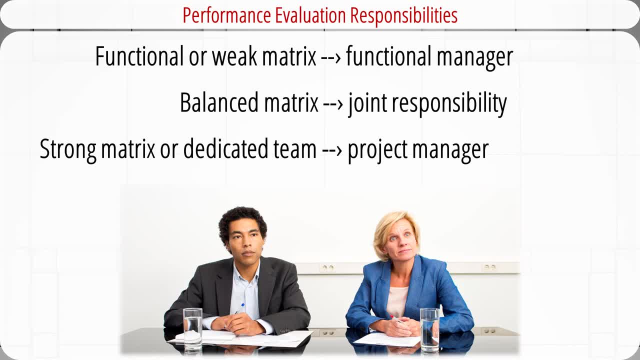 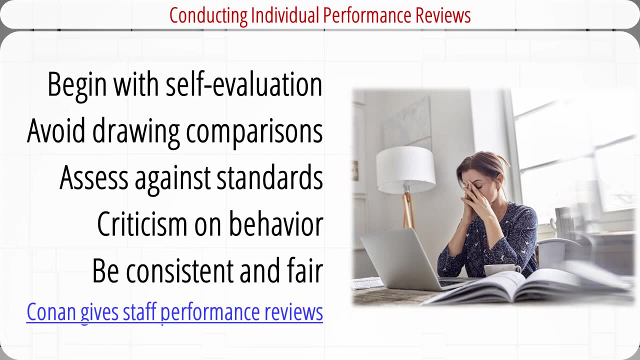 jointly evaluate an individual's performance. When a strong matrix and dedicated team structure is used, then the project manager is responsible for evaluating individual team members' performance. Both managers and subordinates may dread a formal performance review. The process can be stressful and not always pleasant. 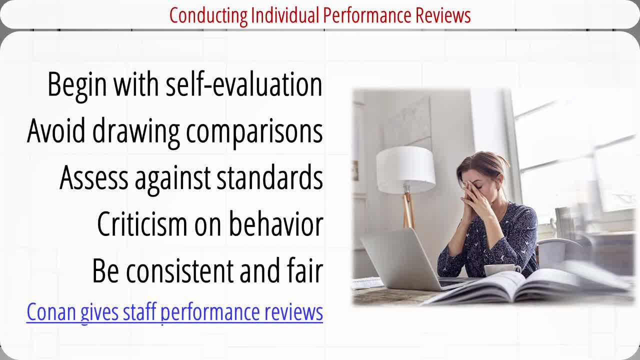 Some good practices are listed here for conducting effective individual performance reviews. The process may begin by asking the individual to evaluate the team member's performance and then evaluate their own performance. When evaluating subordinates, the manager should avoid drawing comparisons with other team members. 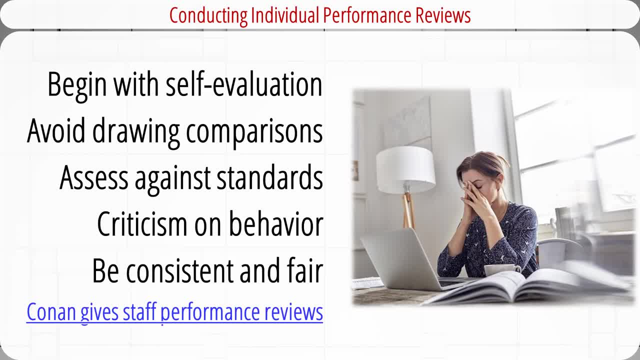 Comparisons tend to undermine cohesion and divert attention away from what the individual needs to do to improve performance. Rather, assess the individual in terms of established standards and expectations. When negative feedback or criticism are offered, the manager should evaluate the team members' performance. 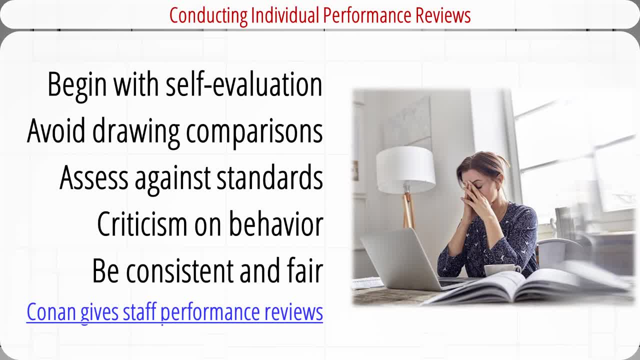 Focus on specific examples of behavior rather than on the individual personally. Describe in specific terms how the behavior affected the project. Also, the performance review process should be consistent and fair in treatment of all team members. Now watch this funny video that shows how the talk show host, Conan O'Brien, gives staff. 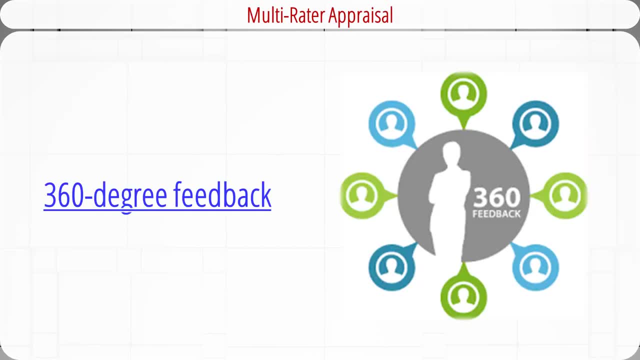 performance reviews. Another individual performance review system is called the multireader appraisal. It's also called the 360-degree review or 360-degree feedback. The review process involves soliciting feedback concerning team members' performance from all the people that their work affects. 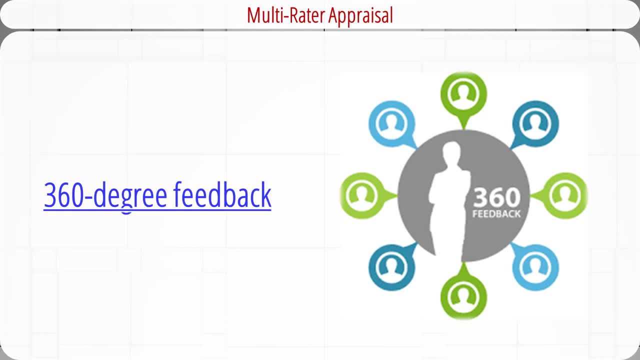 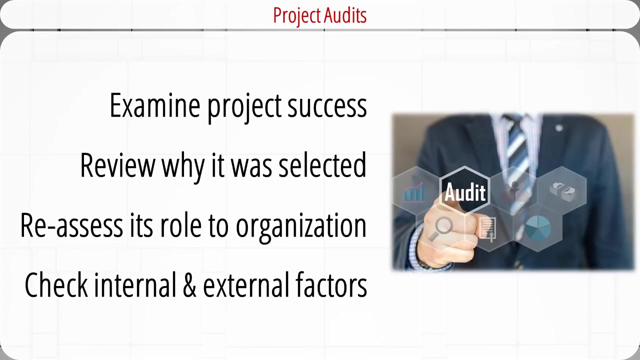 These people include the individual himself or herself, the project manager, the functional manager, peers and staff. This method will provide a more comprehensive understanding of their strengths and weaknesses. Watch this video to see more about the 360-degree review. Project audits are more inclusive than the project status reports and the project final. 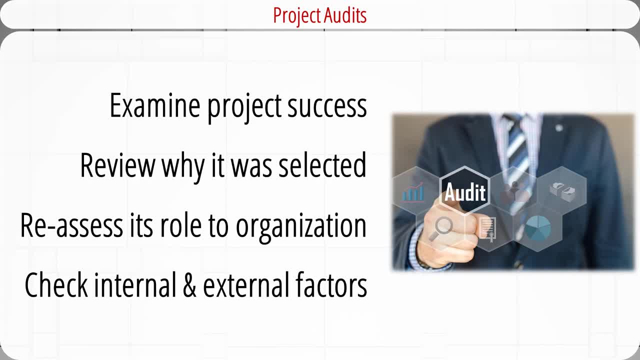 reports. The project reports focus on cost schedule and performance. The project reports focus on cost schedule and performance. The project audits are more inclusive than the project status reports and the project final reports. The projects are more inclusive than the project status reports. 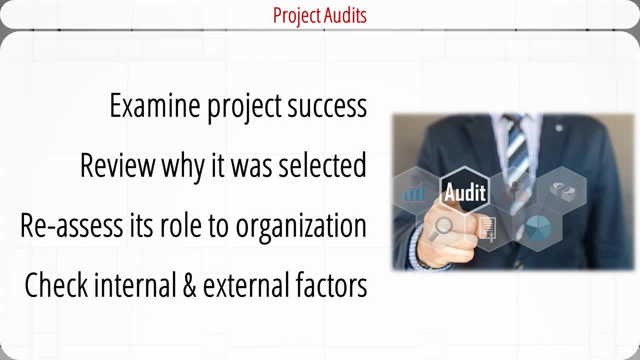 The audits examine project success and review why the project was selected. They include a reassessment of the project's role in the organization's strategy and priorities. They also include a check on the internal factors, such as the organizational culture, and the external factors that contributed to project success. 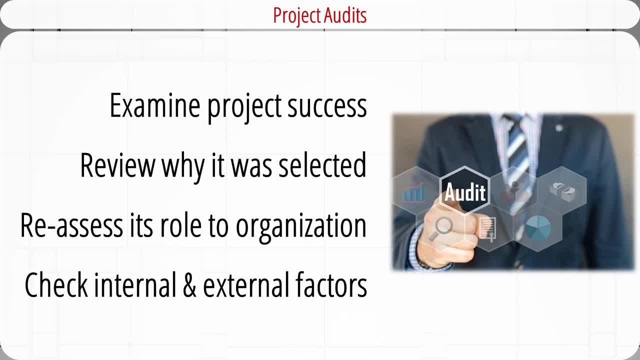 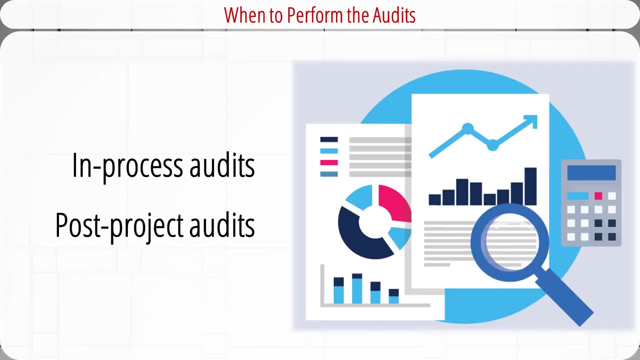 The outcome of a project audit is the audit report. Project audits can be classified into two types, depending on when they are performed. In-process audits are performed irregularly, as the project is carried out. They concentrate on examining project progress and performance. Some early in-process project audits are extremely helpful to allow corrective changes. 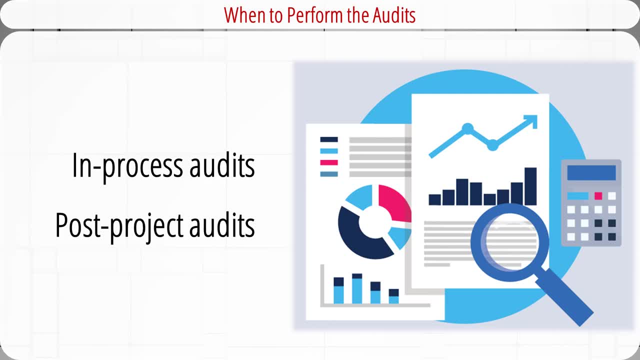 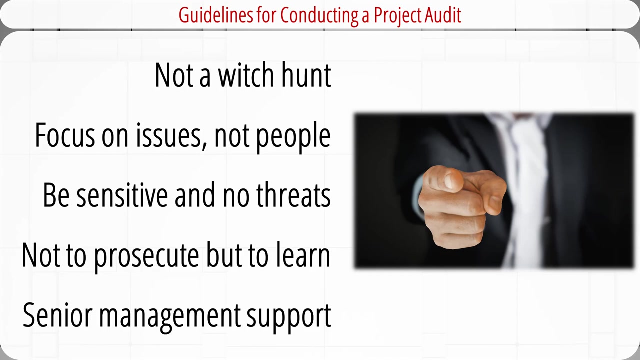 A post-project audit is performed after the project is completed. It emphasizes on improving the management of future projects. Generally, post-project audits include more detail and depth than in-process project audits. Here are some guidelines for conducting a project audit. The philosophy is that the project audit is not a witch hunt. 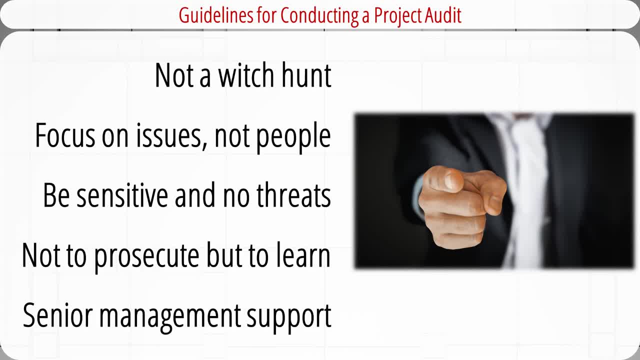 Comments about individuals or groups participating in the project should be minimized. Keep the focus on issues, not people. Also, audit activities should be sensitive to human emotions and reactions. The audit should minimize inherent threats to people being evaluated. Both the auditor and the project team should understand that the objective of project audits 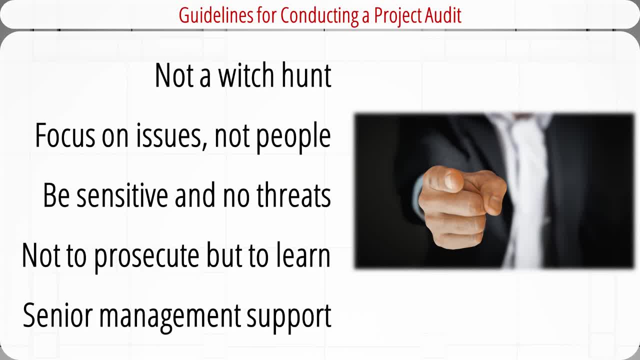 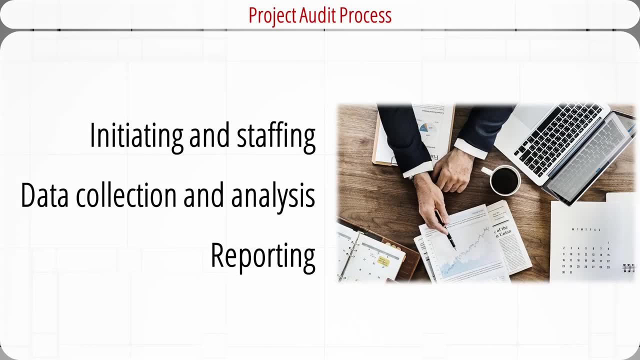 is not to prosecute but to learn from mistakes for long-term growth of the organization. It's very important that senior management should always be aware of the importance of this. Senior management publicly announced support for the project audit to minimize the potential resistance. The project audit process includes three general steps. 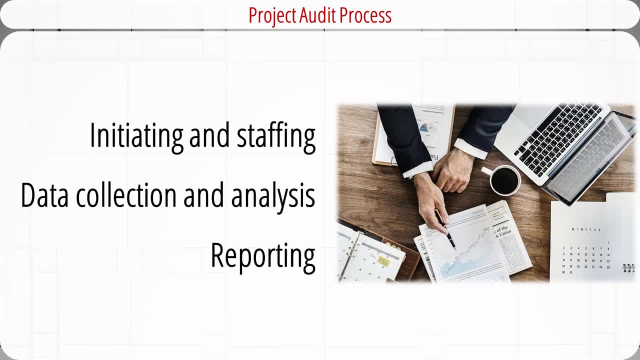 The first one is initiating and staffing. The size of the audit team depends primarily on organization and project size. Also, the people on the audit team must provide an independent outside view of the project. They should have no direct involvement or direct interest in the project, so they would. 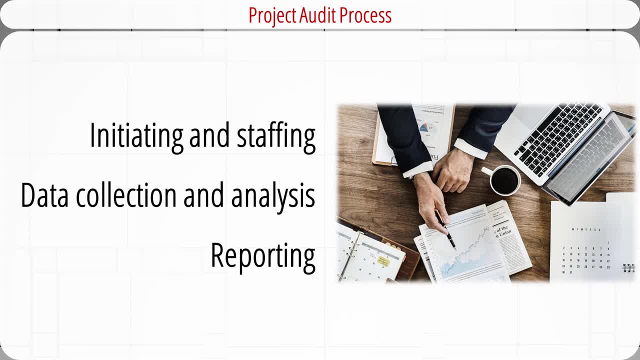 be perceived as impartial and fair. Auditors should be the people who have respect from senior management and other project stakeholders. It's important that they have the independence and authority to report review results without fear of recriminations from special interests. They also must have a broad-based experience in the organization or industry so that they 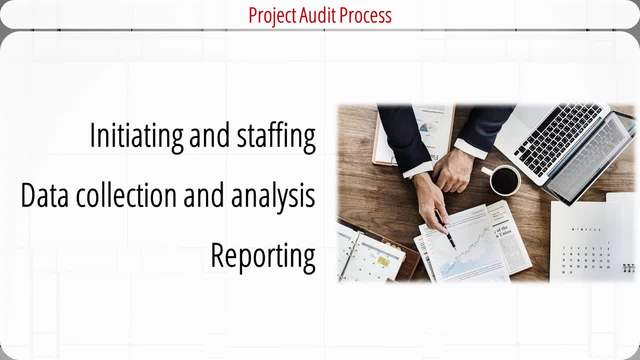 have the knowledge for the audited work. The second step is data collection and analysis. The auditors must gather information and data to answer questions from both the organizational view and the project team's view. The organizational view includes organization culture, alignment, senior management support. 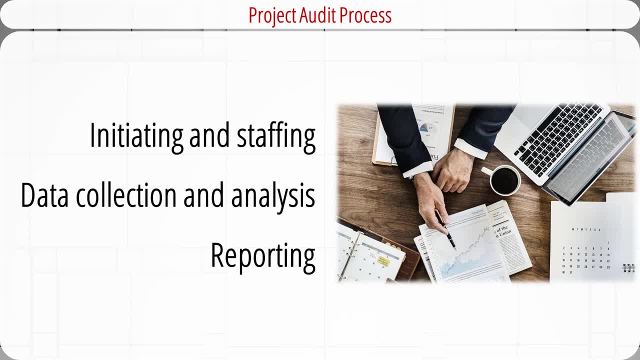 etc. The project team view includes budget schedule, access to adequate resources and the ability to manage the organization. The project team view includes specific tasks, positive or negative team dynamics, etc. The last step is to generate the audit report. The report attempts to capture lessons learned from a current or finished project to improve. 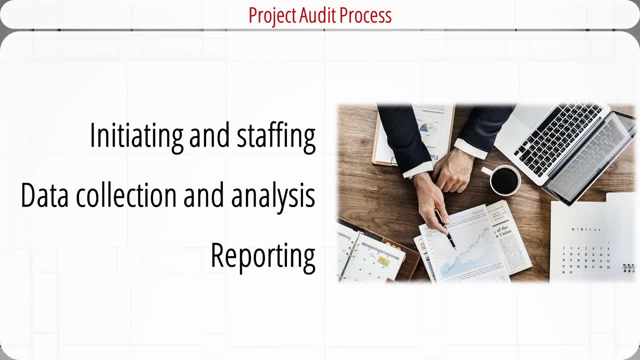 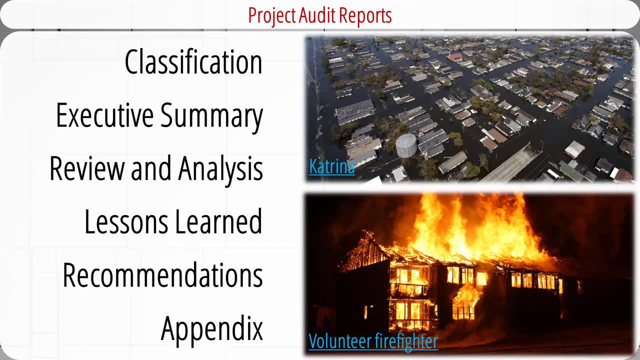 future projects. A project audit report may include the following components: A cover page may tabulate the project information, like the project type- whether it's a complex project or a model project- There is a compliance project, strategic project or an operational project. the project size: 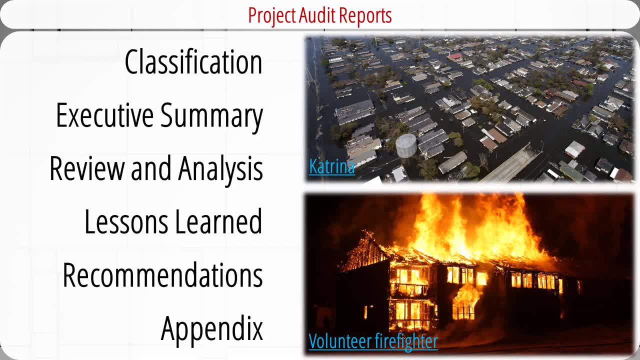 in terms of cost and duration, the number of staff and so on. Then comes the one- or two-page executive summary that simply highlights the key findings and facts related to the project implementation. After that it comes the major part of the audit report, the review and analysis. 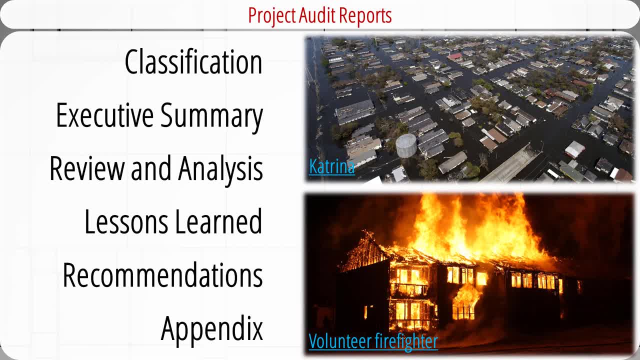 This part lists the project: mission and objectives, technical procedures adopted, organizational resources used and outcome achieved. Lessons learned summarize all the useful tips that are deemed valuable for future projects. They include reminders of mistakes or pitfalls that can be avoided. They also contain retrospectives of actions that were taken to ensure success. 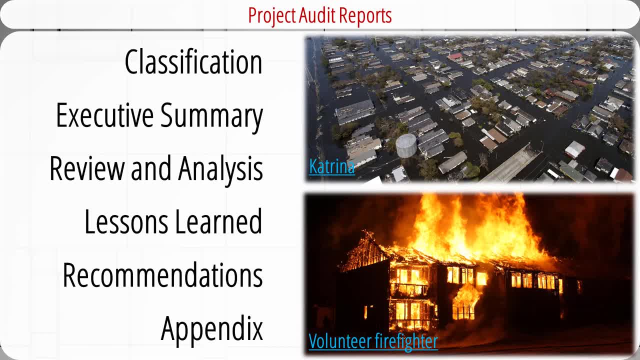 Watch two videos to see some examples. The first video is titled: Five Years After Katrina: Lessons Learned. The second video is titled A Life Lesson from a Volunteer Firefighter, Mark Bezos, who is Jeff Bezos' brother. Jeff Bezos is the founder and CEO of Amazon. 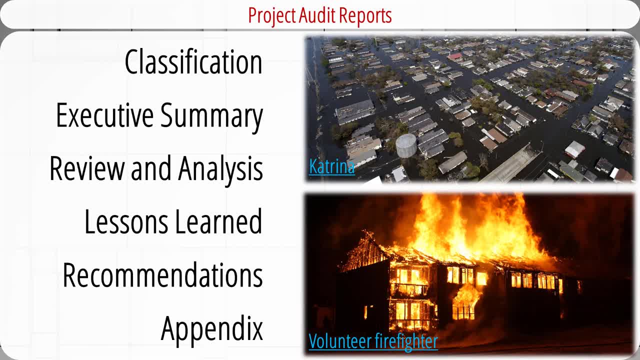 Lessons learned in the audit report are followed by recommendations which include technical improvements. They include updates to the process, corrective actions, etc. Finally, all other relevant but less important information and data can be put into the appendix of the project audit report. 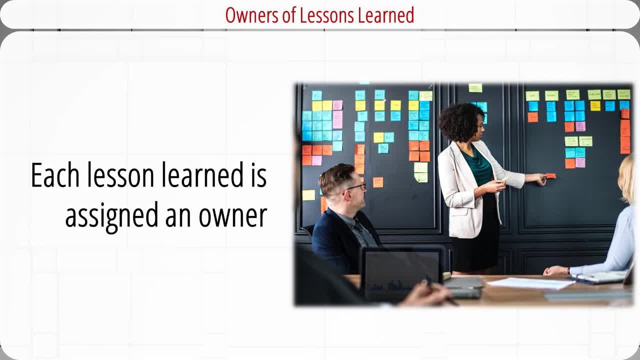 After the audit report is accepted, each lesson learned is assigned an owner. This owner is typically a team member who is most familiar with the lessons learned. We have limited options for each of the two, So some people are more interested in the project. We have limited options for the project. For instance, there are many cases where the project has been quieter than the previous audit report. The second and third cases are: the project is not as active as the previous audit report. The third is the object of the project. 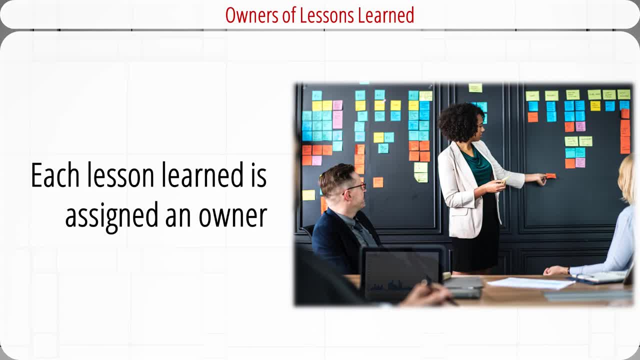 The fourth is the object of the project. The fifth is the object of the project. The sixth is the object of the project. The fifth is the object of the project. anyone who needs information related to the lesson. The owner will assist the documentation and distribution of the lesson, so it will be. 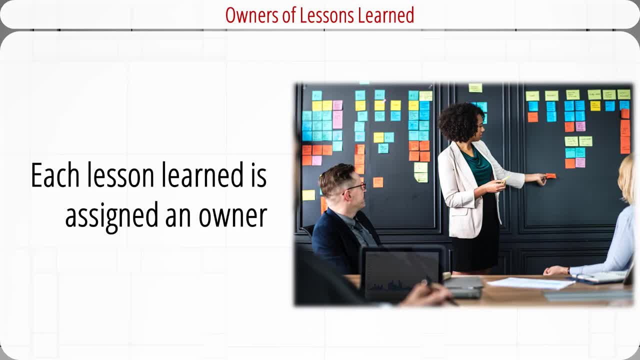 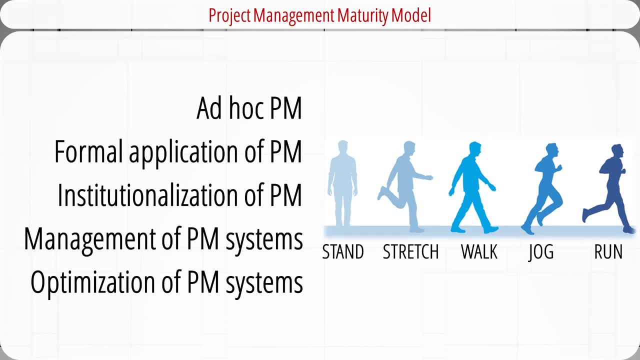 usable by others. Now let's talk about the project management maturity model. A project management maturity model focuses on guiding and assessing organizations in implementing concrete best practices of managing projects. An organization can go through these five different maturity levels depending on how much best practices of project management they have implemented. 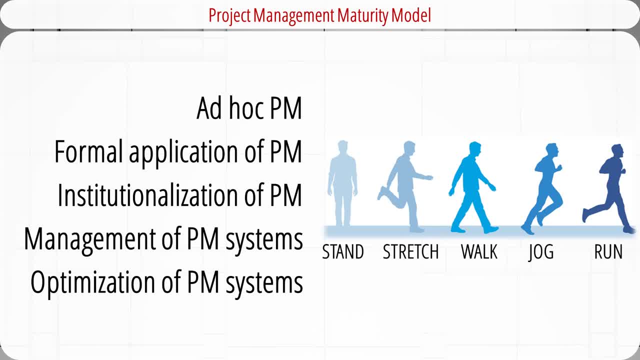 These maturity levels, from low to high, are ad-hoc: project management, formal application of project management, institutionalization of project management, management of project management systems and optimization of project management systems. We can use these five levels of maturity- Use running as a metaphor of these five different levels. 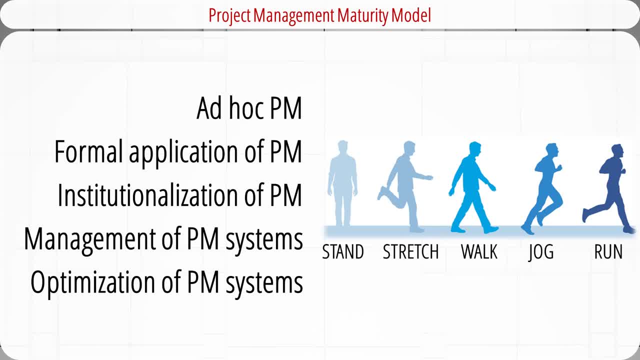 Level 1 through level 5 are represented by standing, stretching, walking, jogging and running respectively. The progress from one level to the next takes time. It could be months or even years. Now let's talk about these maturity levels in detail. 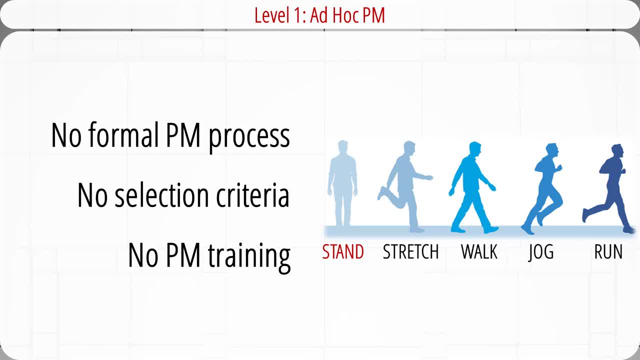 In level 1, there is no consistency. There is no consistent or formal project management process in place in the organization. How a project is managed depends on the individuals involved. If the project manager has project management experience, then they may bring their experience. 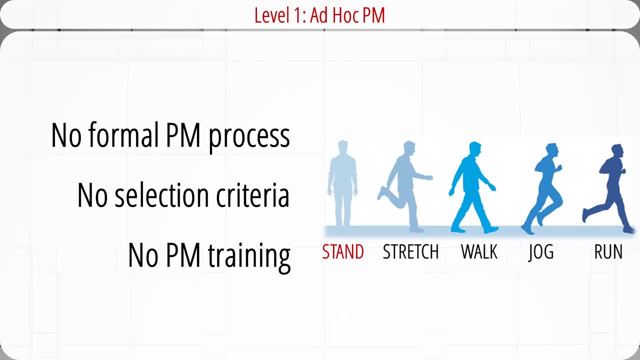 to the new projects. There is no formal project selection system in the organization. Projects are done because people decide to do them or because of a high-ranking manager's order. Also, there is no formal project selection system in the organization. There is no formal project selection system in the organization. 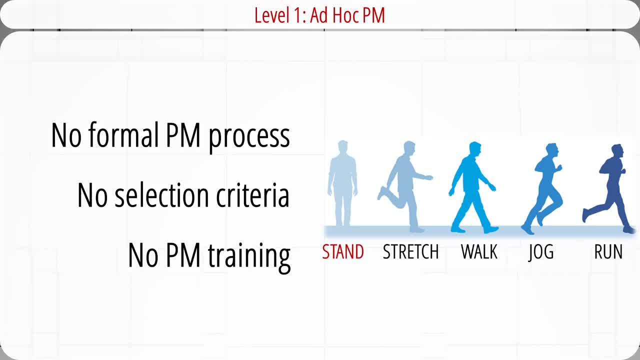 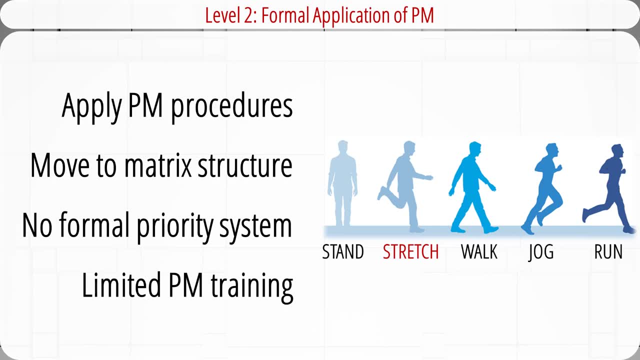 Also, there is no project management training for the employees or managers working on the projects. In level 2, the project managers apply established project management procedures and techniques to their projects: Standard approaches such as scope statements, work breakdown structure and project networks. 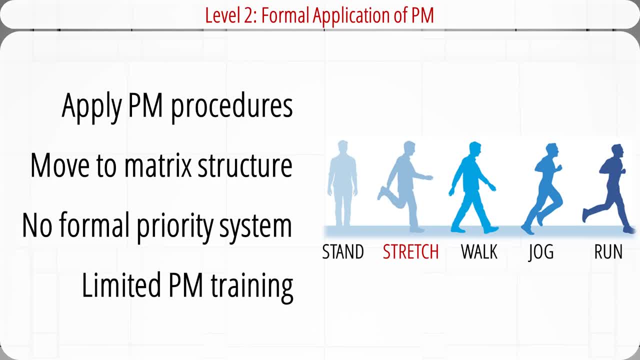 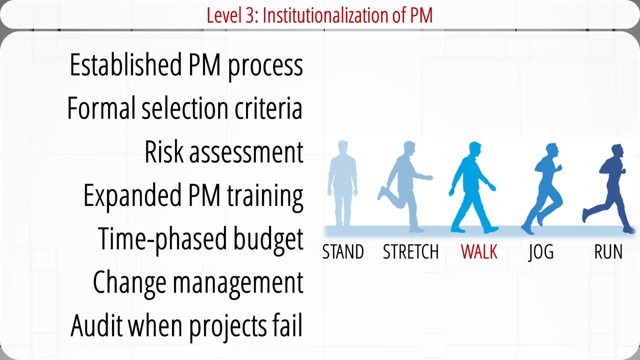 are used At this level. the organization is moving in the direction of the matrix organization structure, But there is no formal project priority system and only limited project management training in the organization. In level 3, projects are managed using well-established process and best practices in the project. 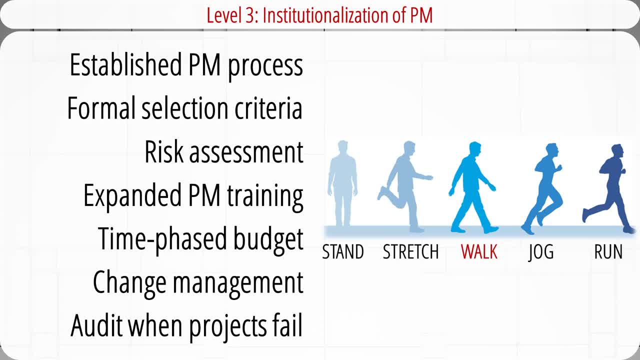 management field. Formal criteria have been developed for selecting projects. Risk is taken into consideration and risk assessment is derived from the work breakdown structure. There are expanded project management training. Time-based budgets are used to measure and monitor project performance based on the earned value analysis. 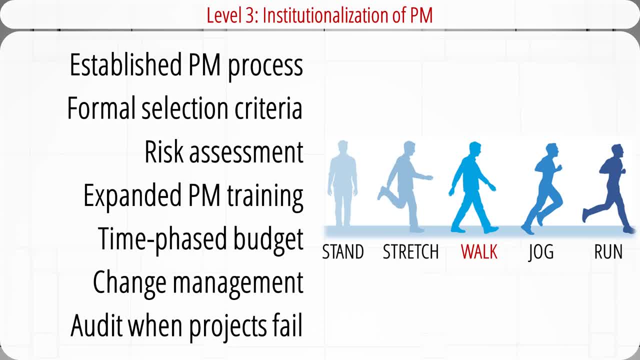 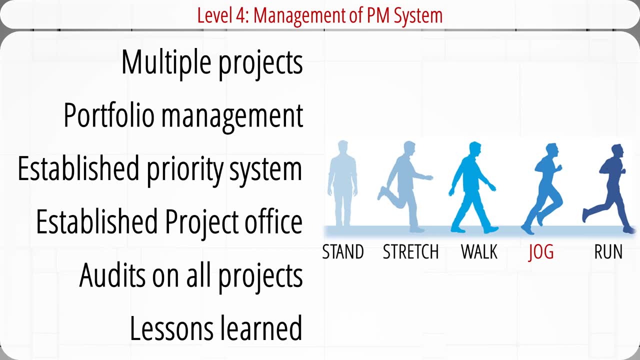 A change management system is in place and all changes are well-documented and justified. Audits are performed, but they occur only if a project fails In level 4, the organization is using a standard system, A standard information system, to manage multiple projects that are aligned with the organizational. 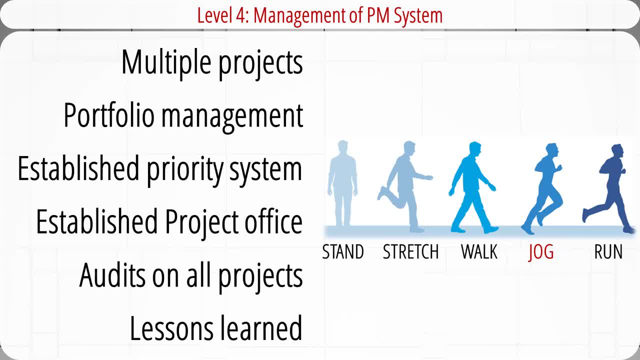 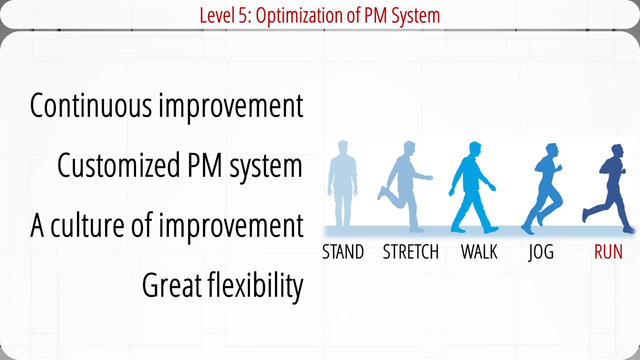 strategic goals. A higher level of management called the portfolio management is in place. The project priority system is established, as well as the project management office. Audits are performed on all projects, Lessons learned are recorded and used to improve future projects. At the highest level, level 5,, the organization is focusing on continuous improvement through 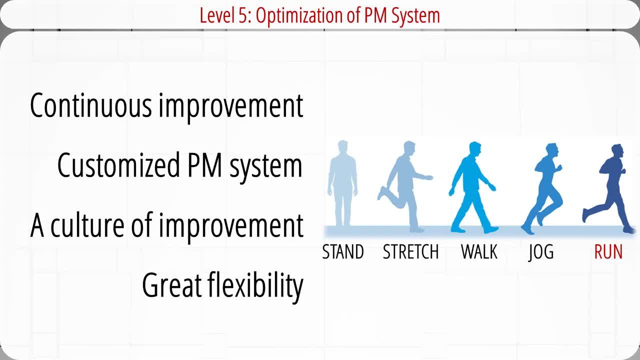 incremental advancements of existing practices and through innovations that base on new technologies. They are not satisfied with the standard project management information system anymore, so they fine-tune and customize them to better meet their own needs. The organization is driven by a culture. They value the improvement.